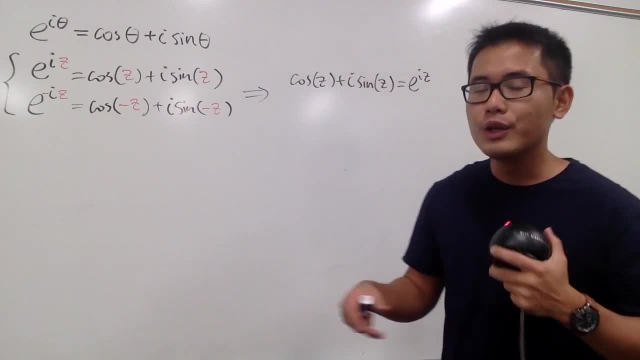 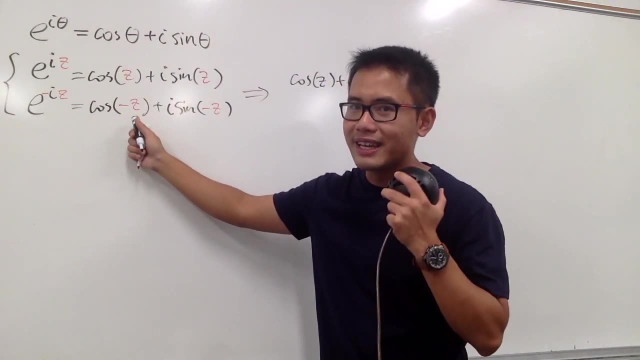 So when you have negative z raised to an even power, you still get the same result as if you have Z inside right. So this right here is even just like the real case. We will have cosine z right here. 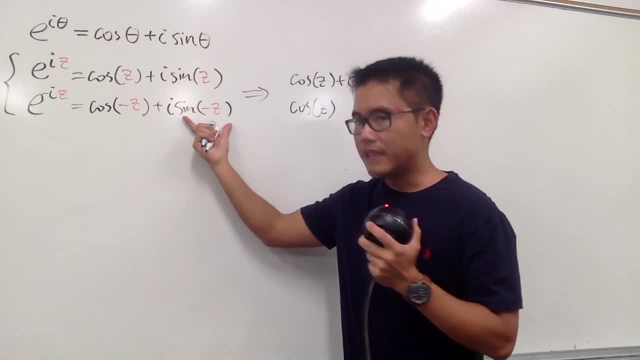 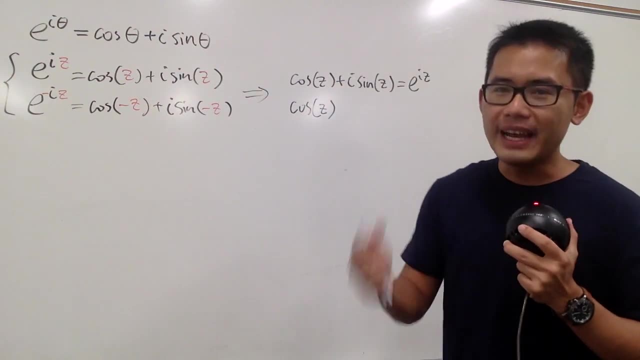 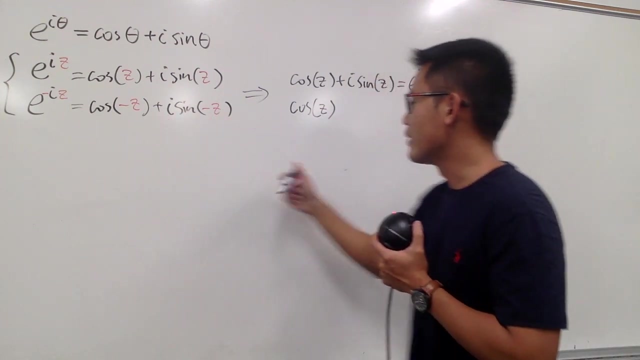 And similarly, when we have sine negative z, this is the same as negative sine positive z, because same thing, Taylor, series of sine. in the complex world you have all the odd powers, so you can take the negative to the front. 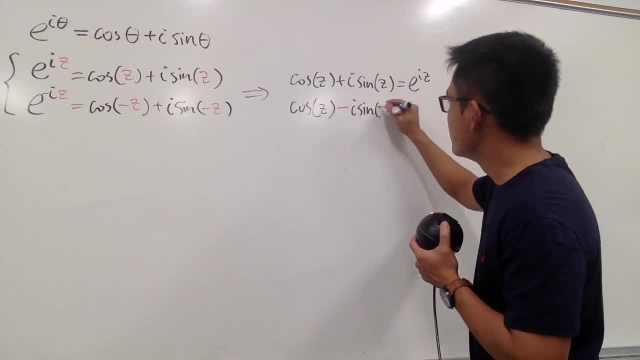 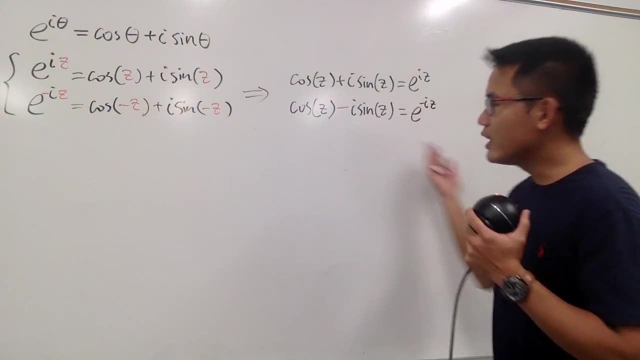 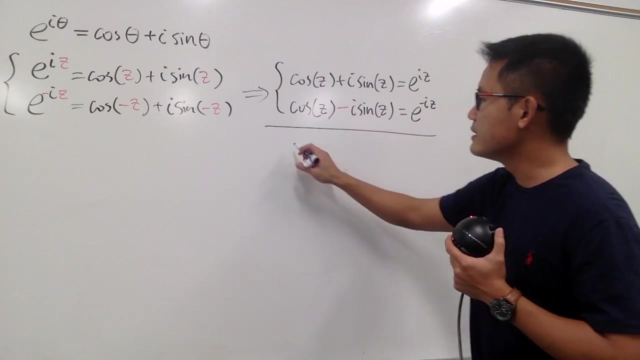 So we have negative i Sine z, And this is equal to that e, to the negative i z. Okay, And from here, what can we do? Well, we can just add these two equations together and you see, they will cancel. and cosine z plus cosine z, of course we get two. 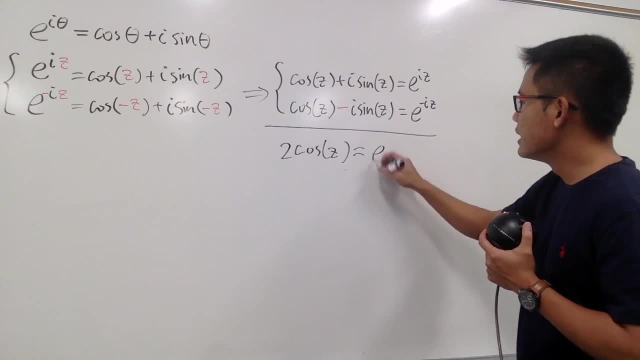 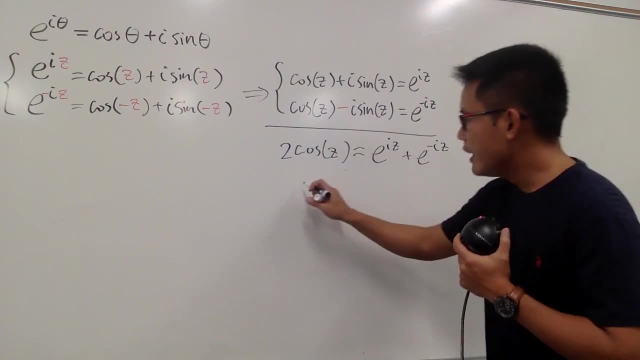 Cosine z, And this is equal to this, plus that e to the i z, plus e to the negative i z, Isn't it? At the end, divide both sides by two, Namely, we will get cosine z equals to. 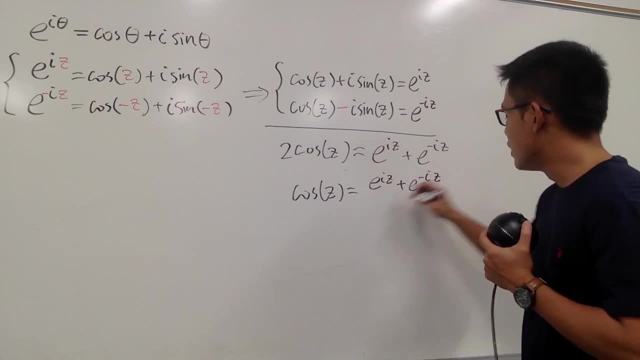 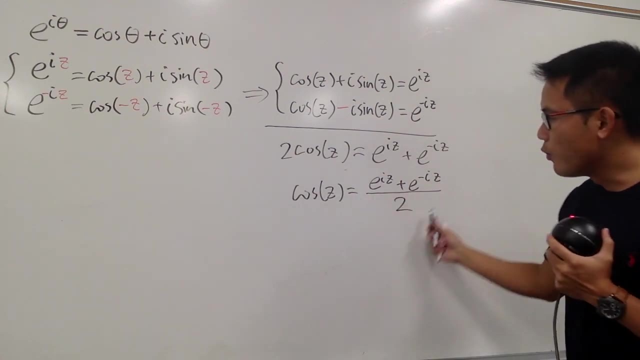 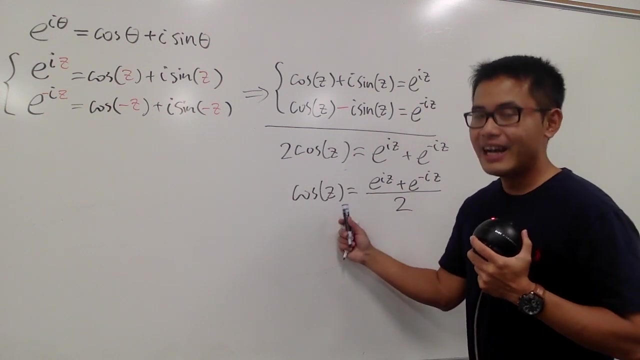 e to the i z plus e to the negative i z all over two. And this right here it's a complex definition of cosine z. Does this form look familiar to you guys? It should, because this is very similar to the cosh x, the hyperbolic cosine x. 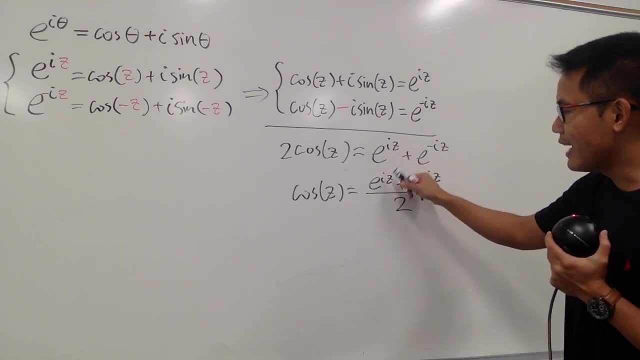 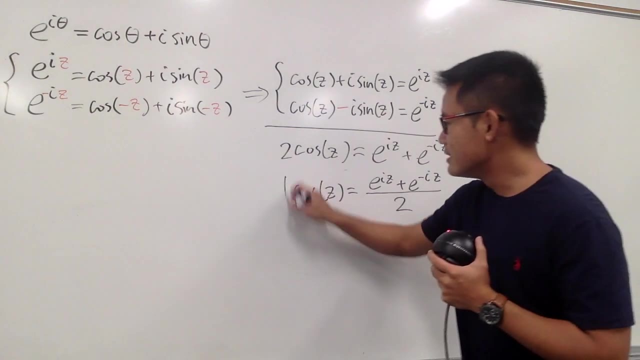 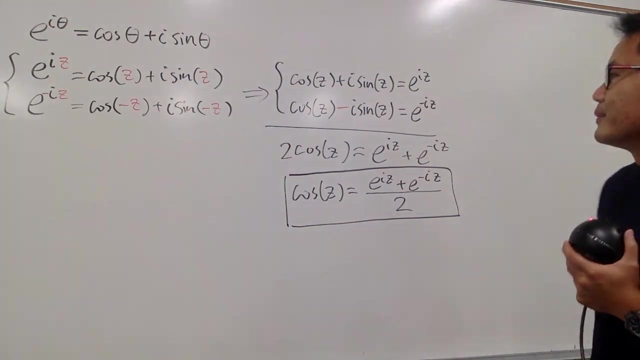 Because hyperbolic cosine x is e to the x plus e to the negative, x over two, right, Really, really similar. So this is the cosine z in the complex world. And now how can we get sine z? Well, we are still going to utilize these equations. 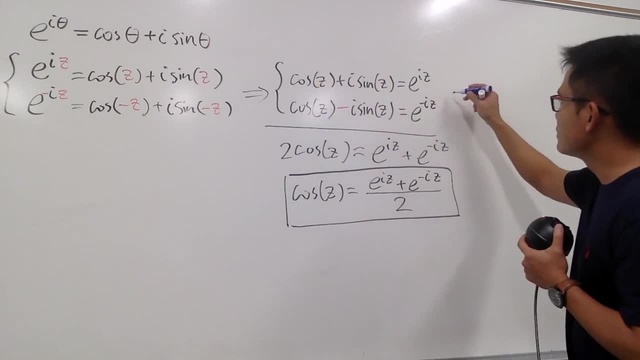 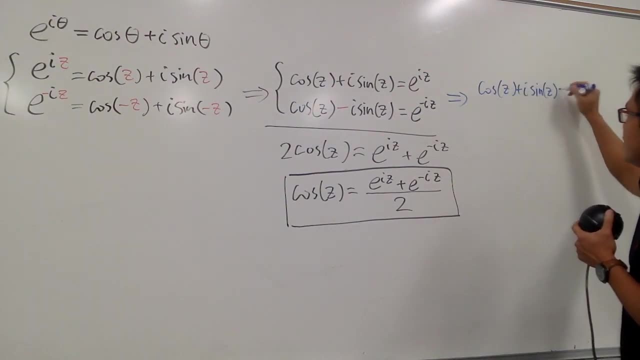 Let's look at this right here. I'm going to keep the first equation as how it is, so I'll do this one in blue. Let me write it down: We have cosine z plus i sine z, equal to e to the i z. 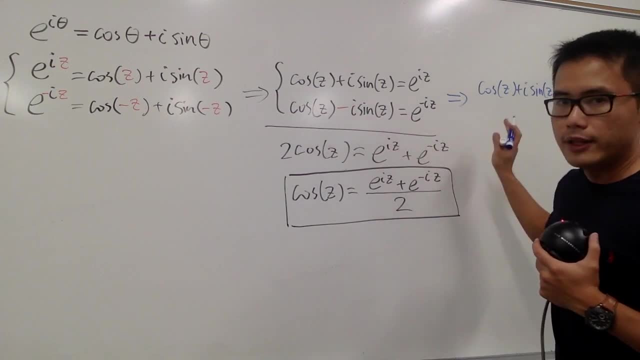 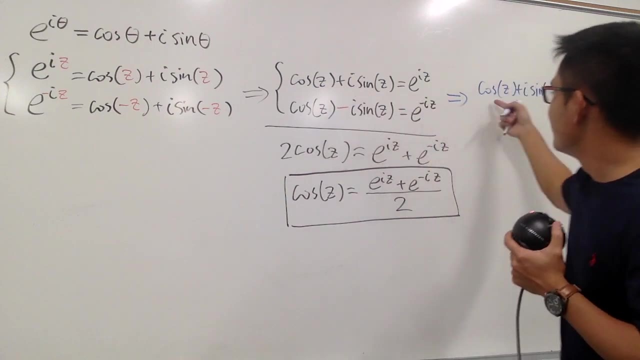 No problem on this? And for the second equation, I'm going to multiply everything by negative 1, so that the cosine z factors will be one positive, the other one is negative, right? So let me multiply negative 1 throughout this, right here.